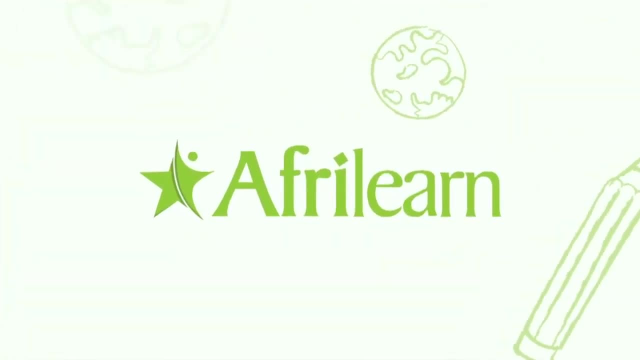 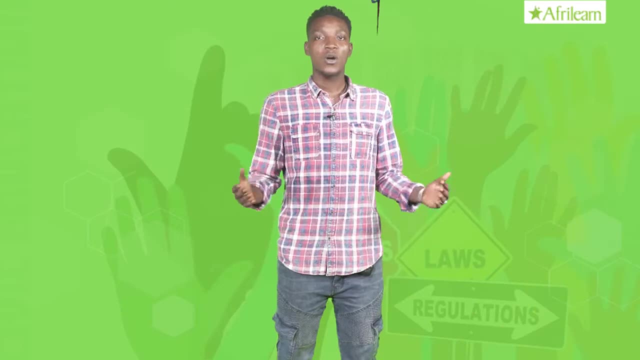 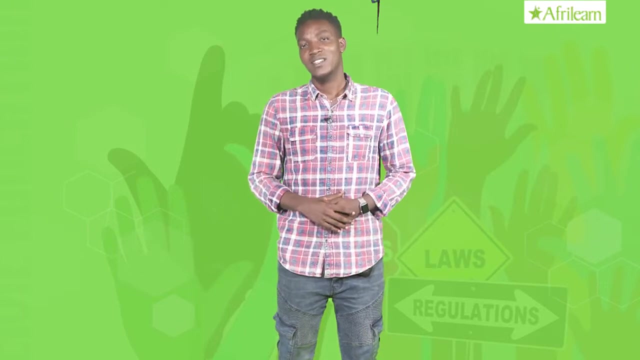 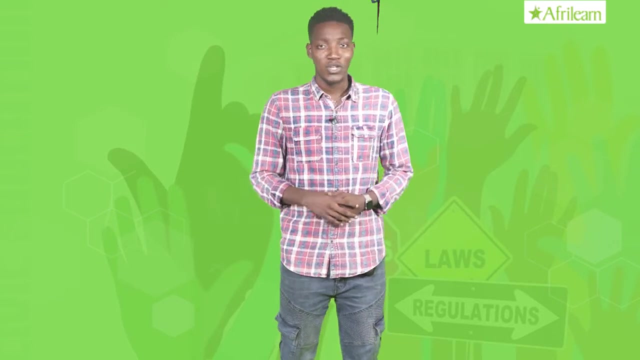 Welcome to class. What is the best thing to do if a classmate slaps you on the cheek intentionally? What if a stranger on the bus steals your mobile phone, Or if your grade in school is reduced because the teacher or instructor doesn't like you? Do you really know what? 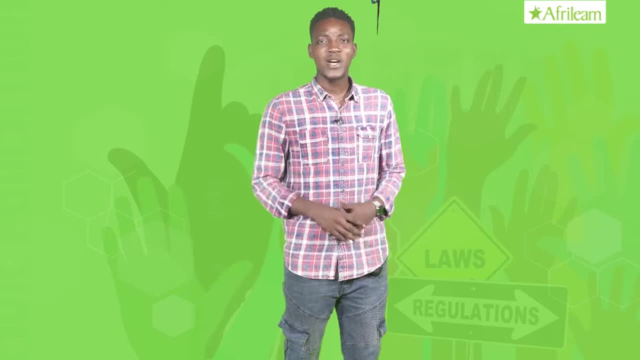 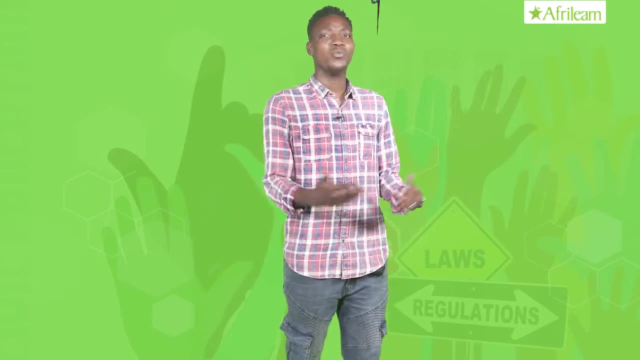 to do As a citizen of a particular country, it is necessary that one must know the rules and regulations of the country, how to get and seek justice, the type of government that operates, how they are elected and how an individual can also be a member of the government. 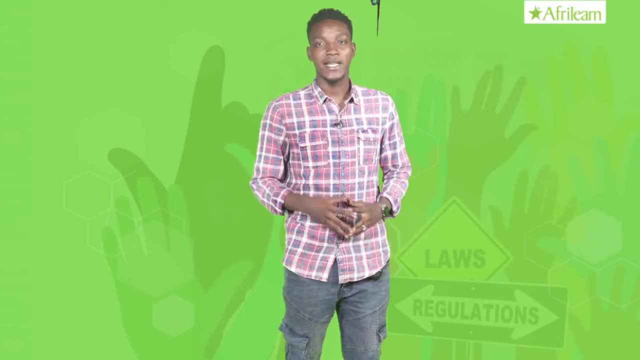 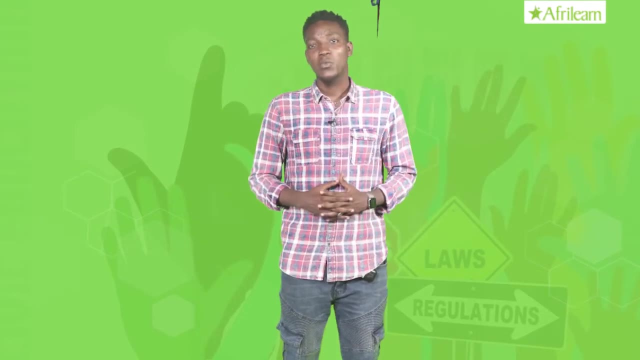 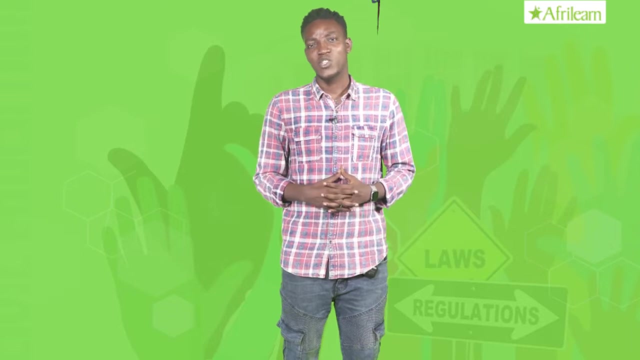 A good knowledge of a subject like civic education would put one at advantage over his peers, because she would know all about your country. This knowledge can make one very responsible because of the values derived from the subjects. Civic education is a subject that discusses the rights and duties of people living in. 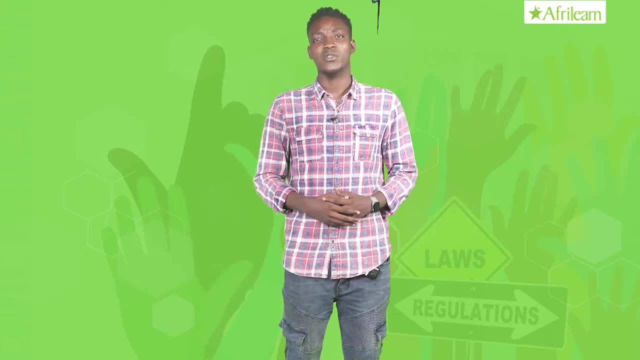 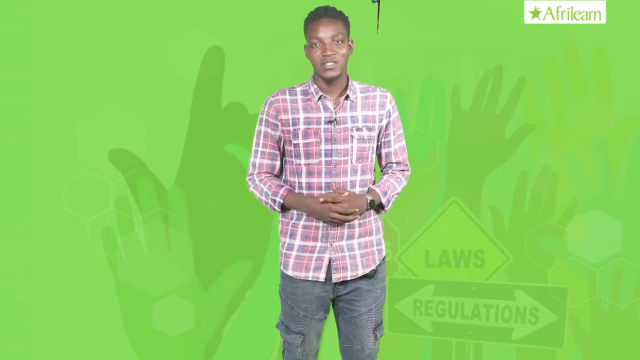 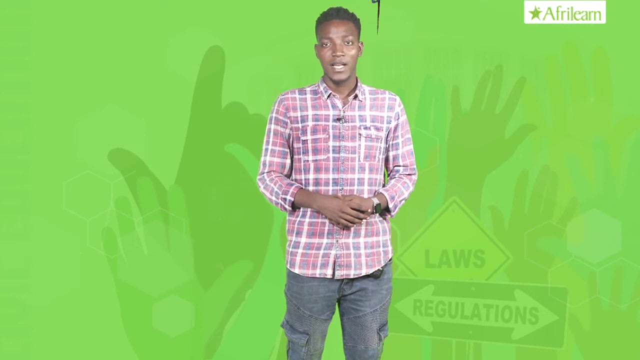 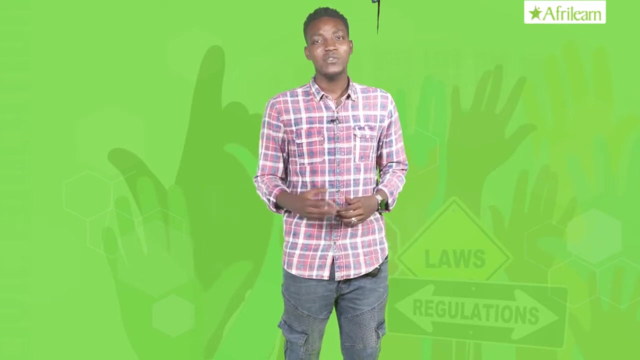 a country, how we relate with family, friends, neighbors and other members of our communities. You can also call civic education citizenship education, because the subject aims at educating the citizens all about our country. This subject is deliberately created to create awareness, teach positive values, right attitudes and behaviors that are acceptable in a society. 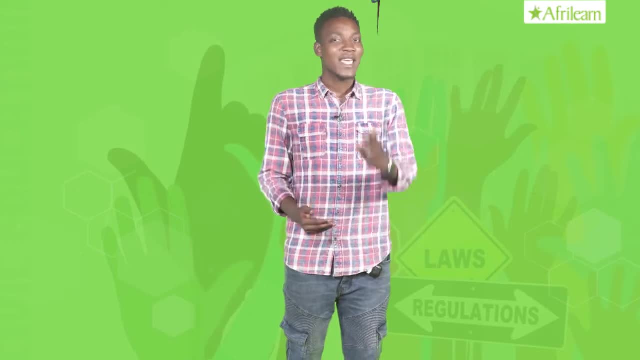 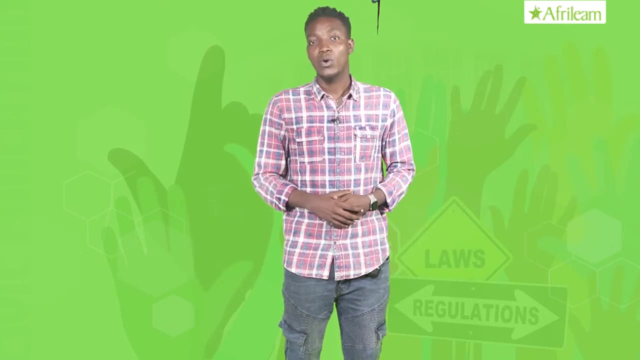 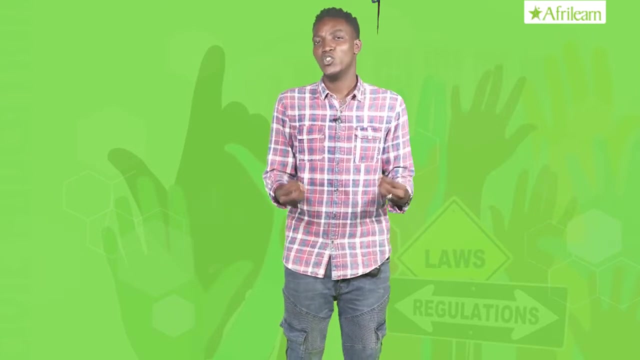 People study civic education for several reasons. For instance, if a teacher decides to reduce your grades because he or she doesn't like you, it is expected that you report to the authorities appropriately. This is instead of you shouting, insulting or disrespecting. 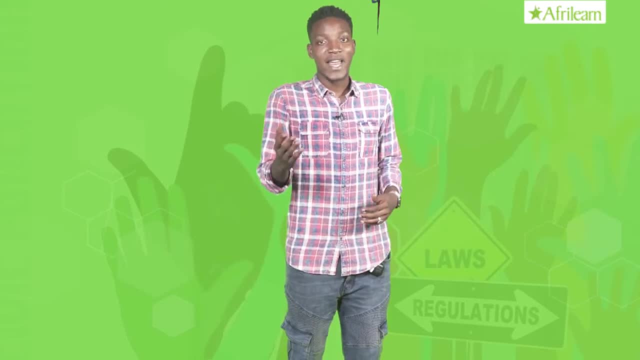 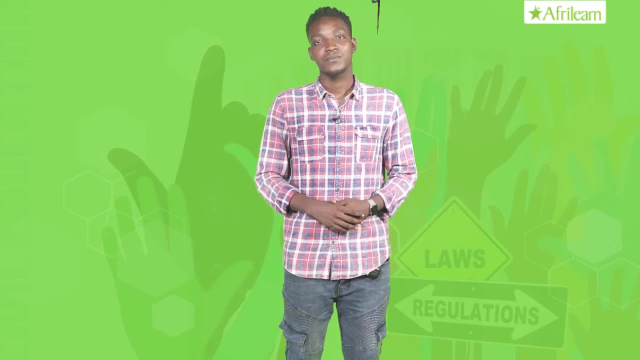 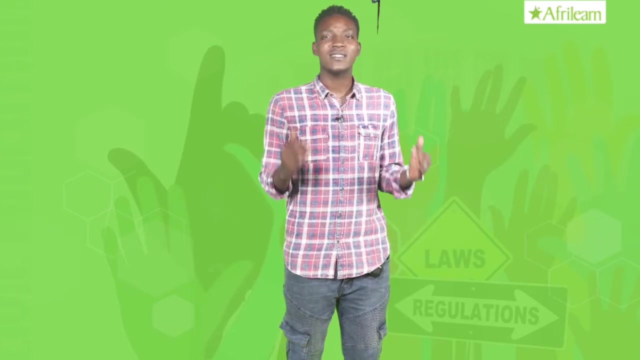 the instructor. You must see the student supervisor or the head of academics or the school principal, depending on the school, to lay your complaint. When you do this, it means you understand your physical and social environment. It means you are civil and do things by the rules and regulations of the country.